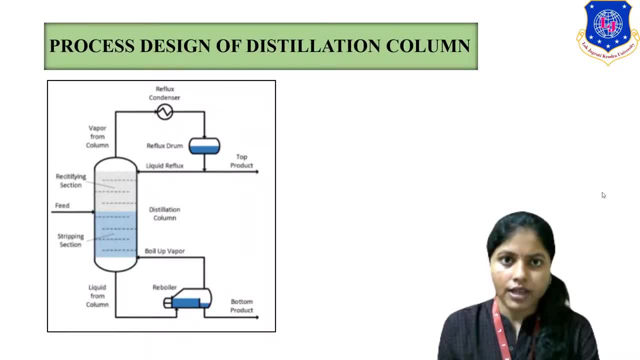 design of the distillation column chapter. in that we are going to see that what are the steps required to design the distillation column. Before going to the distillation column, let us revise the quick revision of the two videos which I have already posted. 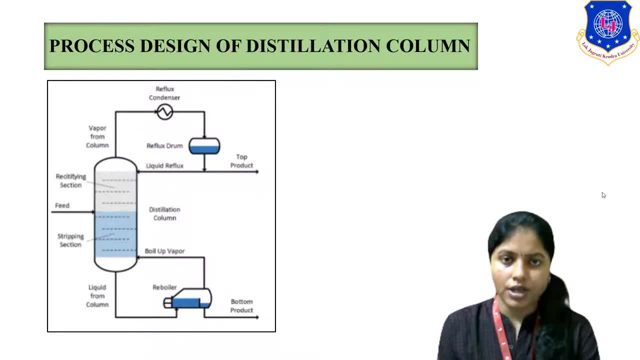 In that video I have shown some of the basics of the distillation column. Second, what is light and heavy key, what are the steps required for the distillation column and what is reflex ratio? So let us go to the figure that what is distillation? Distillation is an liquid-liquid separation. 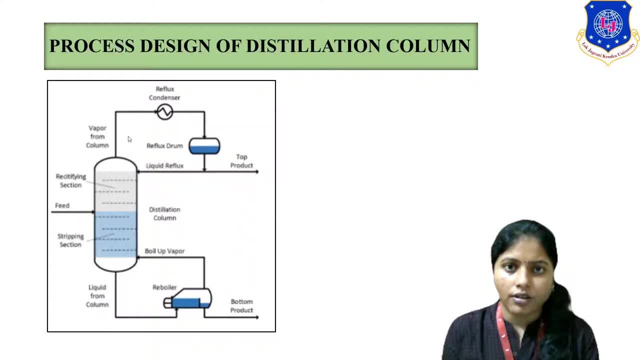 operation which the liquid is being separated on basis on the boiling point. We have to see over here that the separation should be based on the boiling point. So what happened over here? that the feed will come into the column and the more volatile component will go into the condenser and 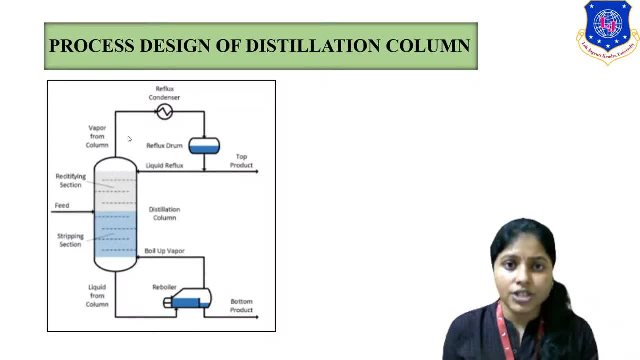 it will form a distillate. The distillation is denoted by D, While the lighter or less volatile component will go into the bottom part and it will go to the reboiler and form a residue. It is denoted by R or W. in there are two parts: rectifying part and the stripping part. The feed above the. 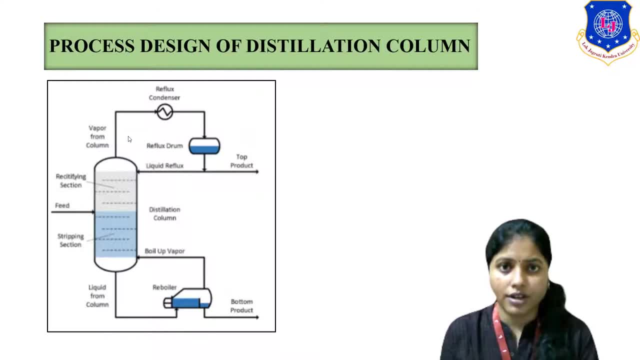 section is known as a tap sent. The feed above the feed is called as the tap and it will be connected. rectification or the rectifying section. The feed below the section is known as stripping section. So what happened over here in the rectifying section is that 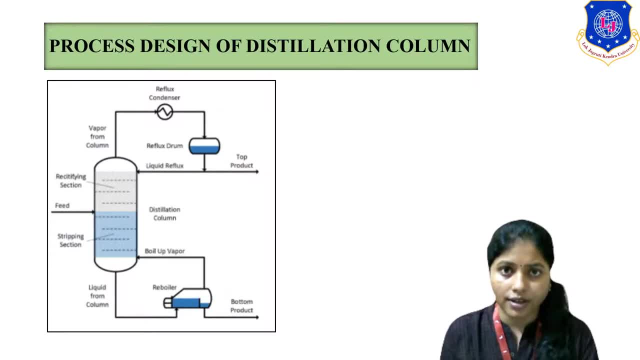 when the feed comes to the condenser and it will condense the vapor into the liquid form, it will go into the distillate, but some part of the distillate will reflux back through the reflux drum into the column. This will help to increase the purity of the product in the distillation column To 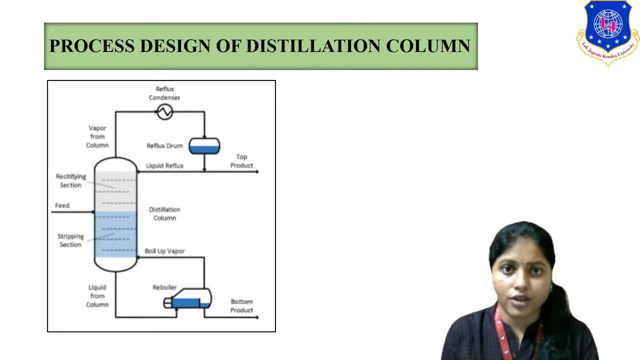 increase the purity, we have to ensure that the total reflux is done when the distillation column is at the starting phase. Then we have seen the two components, that is, Like key and the heavy key. So what is Like key? Like keys, a Component which, in the distillate, will pour electric current into the column When the distillate is. 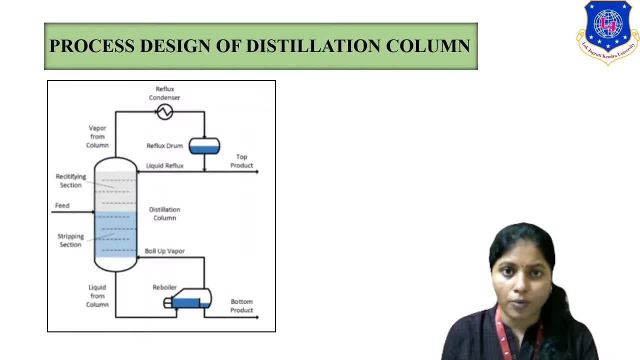 component which has more volatile component and it will pass through the condenser, While what is heavy key- The heavy key- is the component where it has less volatile component and it will pass from the reboiler and it will pass through the stripping section. It will pass through the 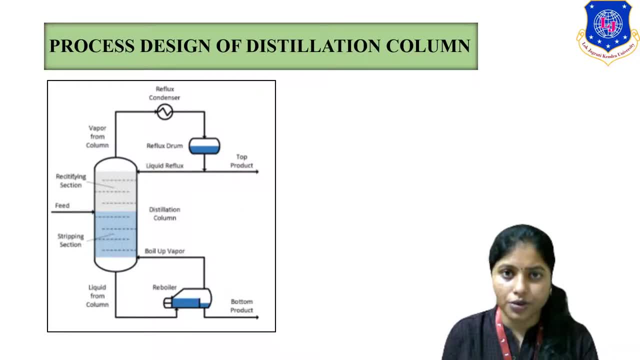 stripping section. We have also seen the reflex ratio. So what is reflex? Reflex is passed from the reflex drum, where it will take some part of the distillate into the column or it will reflex back into the column. It is denoted by R and it is given by R is equal to L, by D There are 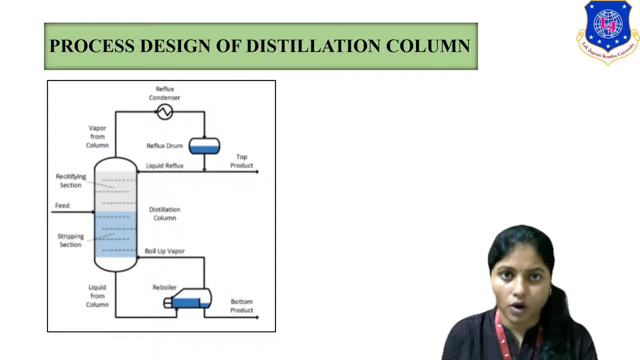 three types of reflex: Total reflex, optimum reflex and minimum reflex. In the total reflex, what it happens? that the no distillate is taken. Full total distillate of the product is been coming back into the reflex, So the distillate will be zero. So R. 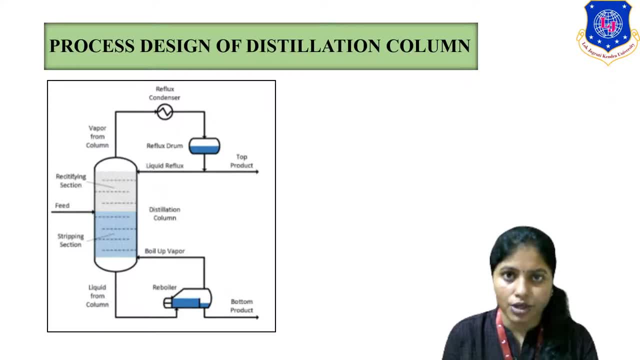 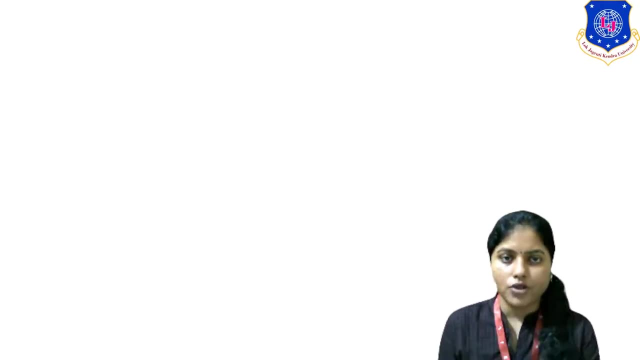 equal to L, by D, So D, that is zero, So R equal to L, which is infinity. So we need here 0. A lot of stages or the lot of stairs separating stages in the column. So we will start with the today's video, that with the sixth topic, that is, type of tower. There are two types of tower that. 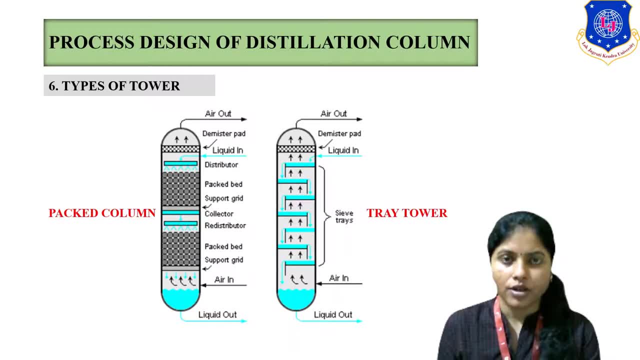 is tray tower and pack tower. So in this figure you can see that what is tray tower? Tray tower is a tower where different type of trays or plates are being placed in the column, While the pack tower is that the packing material is placed between the column. Let us see in the figure. 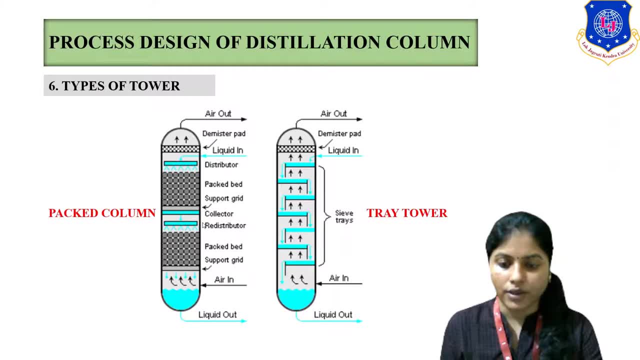 Let us start with the tray tower. In the tray tower what happens? that when the liquid is coming or the feed is coming in the side, the column, then it will pass with one of one tray to the second tray or the third tray, And it goes on. But we have to see different things for the mass transfer operation of liquid and gas. So the liquid is coming from the top and the gas is coming from the bottom. 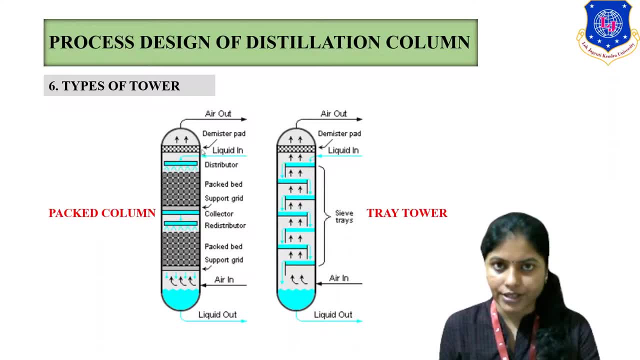 So what happen over here? that when the liquid enters, It has the weirs, known as it will hold up the liquid in the tray And you can also see the extension of the weir that it is known as downspout, which means it will help the liquid to pass or to move to the second tray. 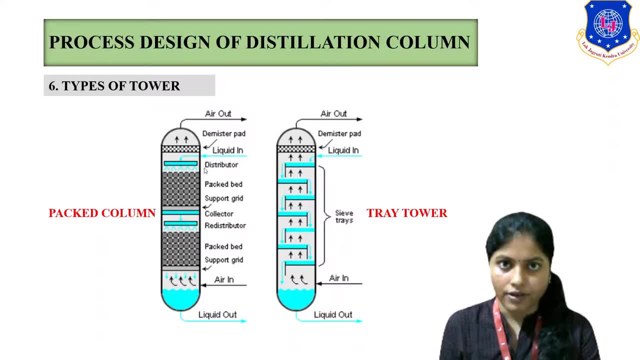 This all will help the tray tower to have the good efficiency, or the good efficiency or the good mass transfer between the liquid and the gas. So this- I have shown the figure of sieve tray, While what happened in the packing column is that the liquid is coming from the top. 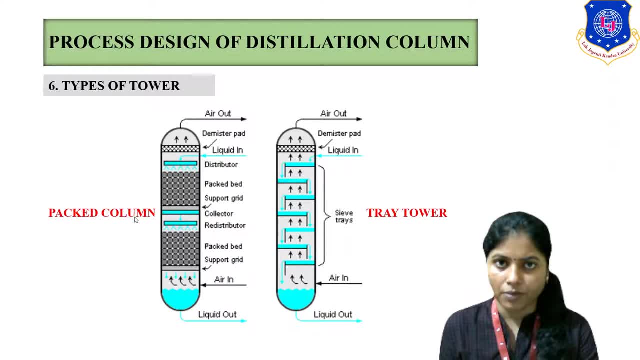 and the air or the gas is thrown from the bottom. Here the liquid distributor is kept on the top of the column. Here the packing material is been placed between the column. So what happened over here? that when the liquid comes from the top and the liquid distribution has been taking place. 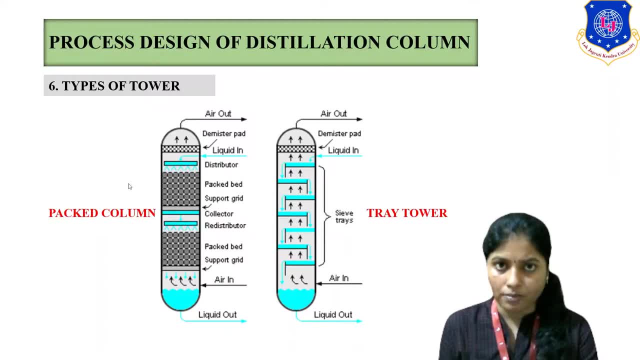 then it will pass to the packing column. That packing column will ensure that the mass transfer is taking place between the liquid and the air. Here we have also placed between the redistributor or the liquid distributor again, because if we don't keep the redistributor in between the column, 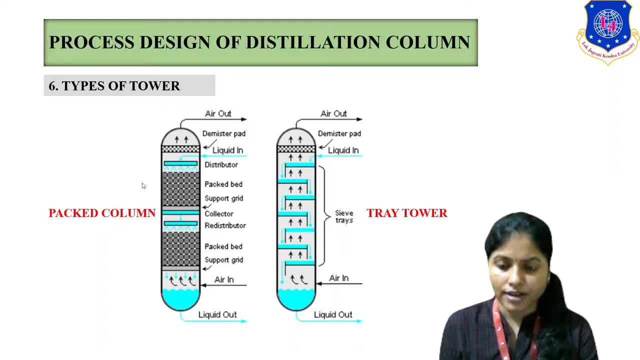 then the channeling problem will be there. Channeling problem. Channeling means the liquid and the gas movement or the flow will not take place between the packed column. It will go by the side of the column. I repeat, it will go on the side of the column. 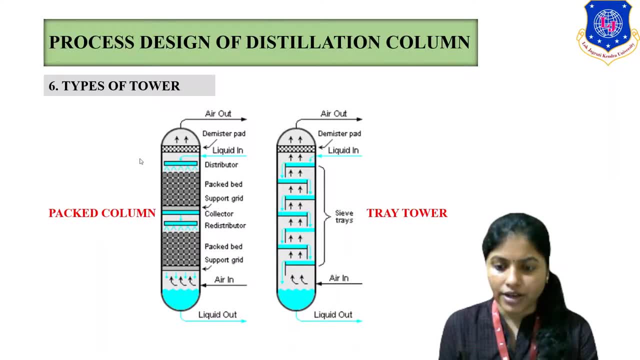 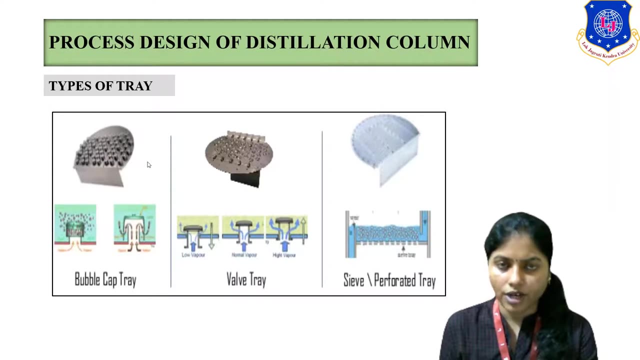 So that problem is known as channeling problem On. there is support grid, seen in the figure. Support grid is nothing but the grid kept for the support for the packed column Moving it. with the types of tray, There are three types of tray: Bubble, cap tray, valve tray and sieve tray. 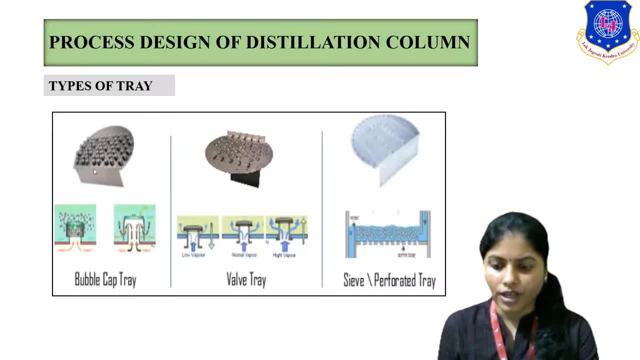 In the bubble cap tray. what happened over here? when the gas is been flown from the bottom or the vapor coming from the bottom With the help of the vapor intensity or the vapor will ensure that it will open the bubble. We will be able to see the rubber fully visible too on there. 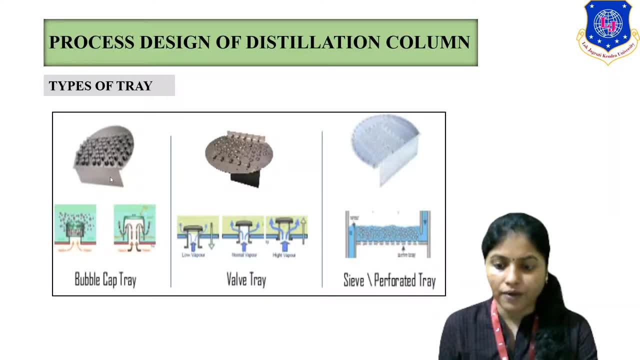 Or the The speaker will have some light beam. We will Can See Here That. Or Or The Whistle. You can see in the figure that the upper part, it will get blown on and the liquid and the gas mass transfer will take place, While in the valve tray- what happened over here already- ​the valve has been kept on the top of each of the trays. 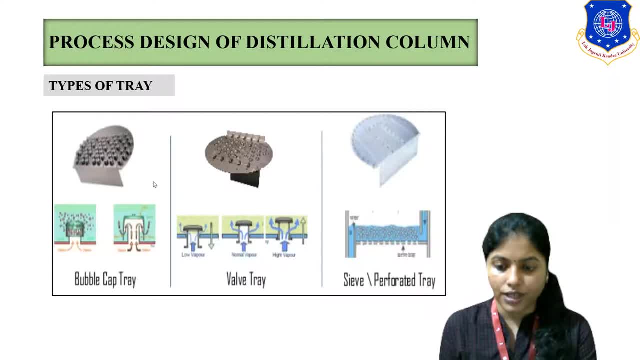 will pass from the side of this side of this liquid and the gas of the valve, and the mass transfer will take place while what happened over in the sieve tray, that the holes is been placed on the plate tower, and from the holes the liquid and the gas will come in contact. 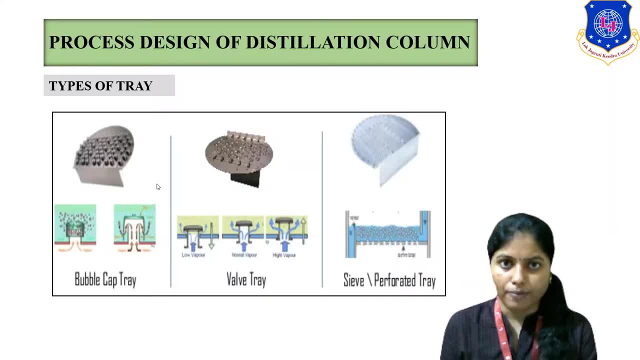 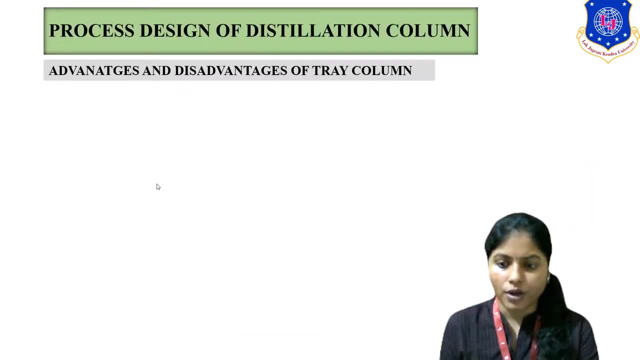 with the each other and it will help for the better absorption or the better separation. so moving it with the advantage and the disadvantage of tray column. the advantage is it is cost effective, can handle high liquid flow rate and the disadvantage is high pressure drop in pack column and foaming can occur during education. 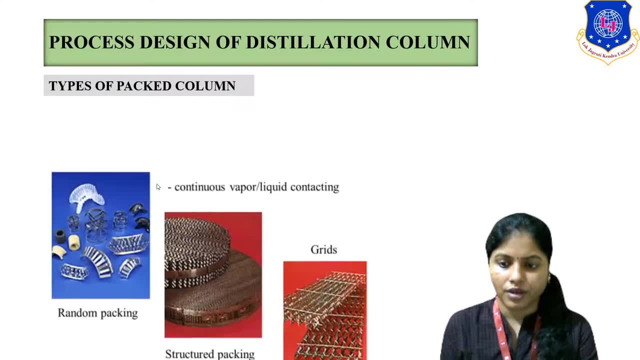 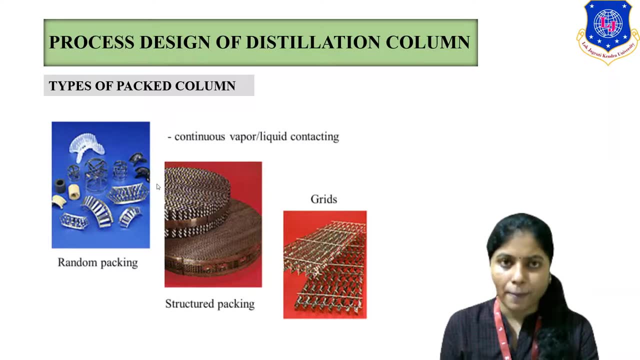 the types of pack column. there are three types of pack column, but mainly two are been considered: random packing and regular packing. so what happened in the random packing? in the random packing, the random type of beads are been placed on the column. so the packing material. then, after using the media, press the cryouria bags. and where do the differentZe big الم? 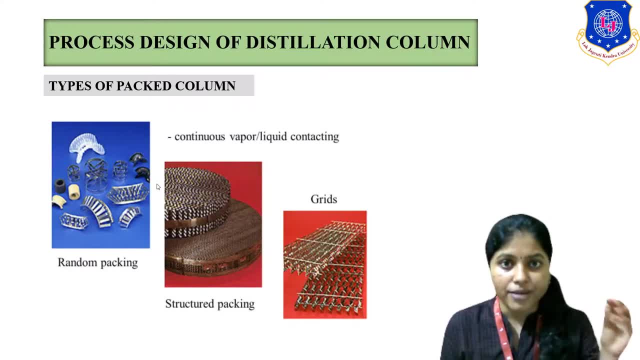 used in the pack column are of random shape, So that is known as random packing, While in the regular packing the regular, the similar type of or the uniform type of packing material is being placed in the packing column, So that is known as regular packing. 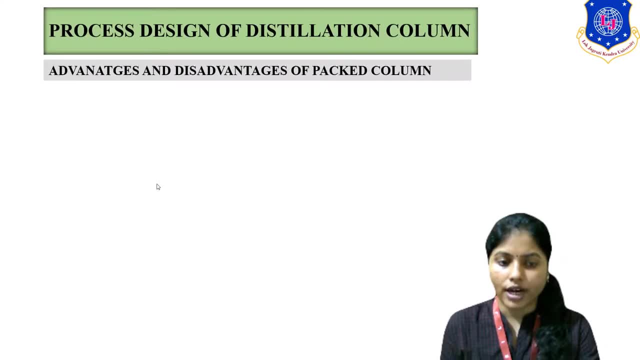 Moving ahead with the advantage and the disadvantage of the pack column. The advantage of the pack column is direct injection into the column, large solute capacity, While the disadvantage of the pack column is it is less retention time and it is very costly. Moving ahead with the difference between pack and pack column. 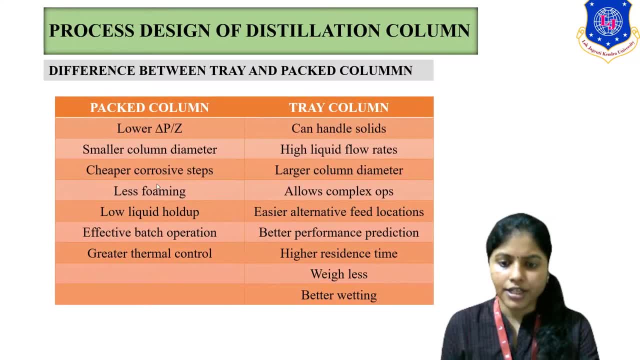 It is mostly asked in the exam point of view or the interview. The pack column- we can see it- has smaller column diameter. It is cheaper but for the corrosive steps It form a less forming than the tray column. It has low liquid holdup. 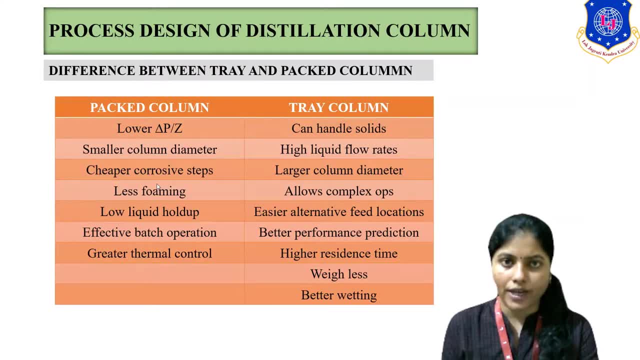 It also has the effective batch operation and it also has the greater thermal control. While in the tray column it can handle the solids, It will have high liquid flow rate. It has the larger column diameter. It form an easier alternative feed location. 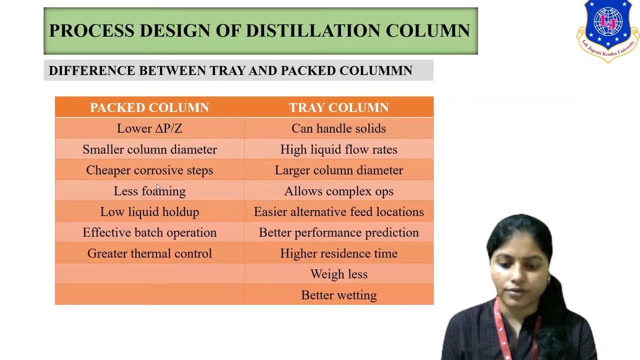 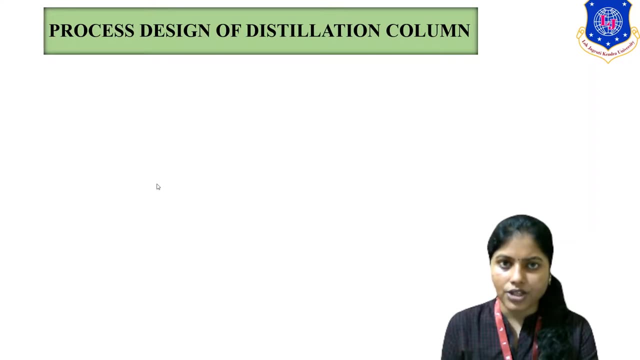 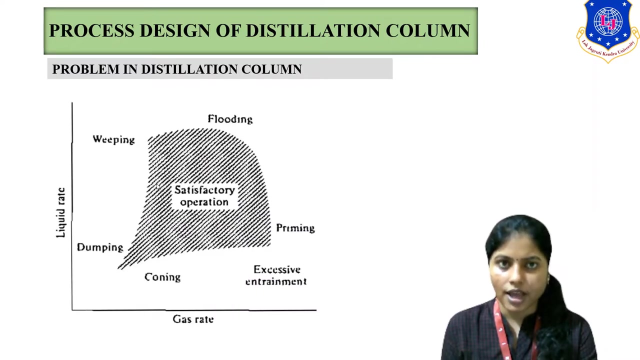 It has better performance. It has better performance production, It have higher resistance time, Its weight is less and it has better wetting power. So there are some problems in the distillation column. The problems in the distillation column are shown in the figure. that is weeping dumping. 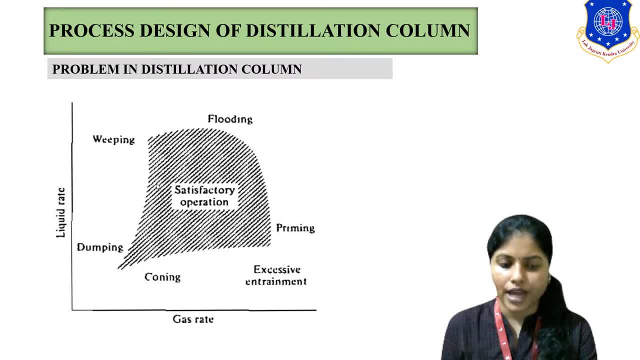 flooding, priming, excessive entrainment and coning. So in the X axis we can see the gas rate, while in the Y axis we can see the liquid rate In the coning. what happens? that the low liquid and the low flow rate is been there. 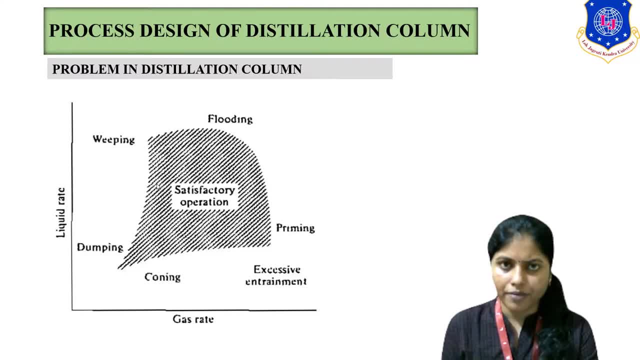 So the coning will take place, while in the entrainment, high vapor flow rate and high liquid flow rate will be there. In flooding, high vapor flow rate and high liquid flow rate will be there. In flooding, the high liquid and the high vapor flow rate will be seen in the flooding. 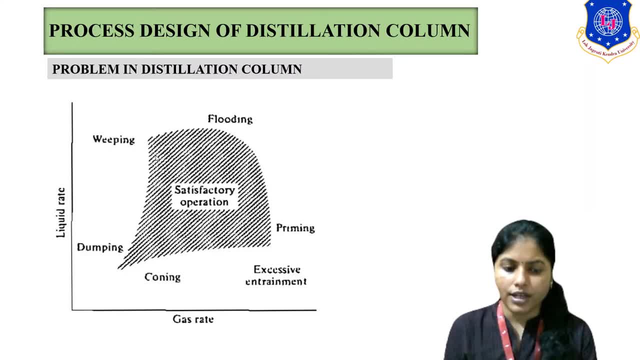 problem. So what happen over here is that when it has an high liquid in the column and a high vapor flow rate, the liquid will starts to pour from the each strain Right, So it will form a flood type of situation. So it will form a flood type of situation. 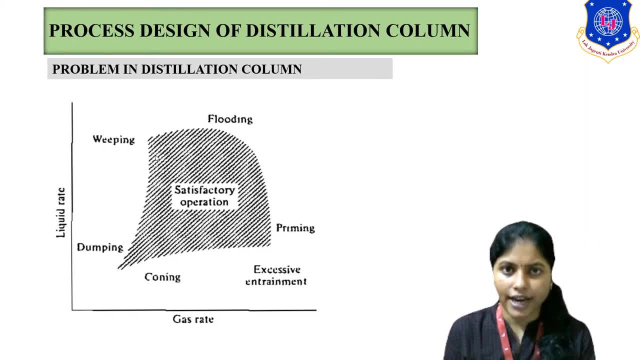 So it will form a flood type of situation In the column, while in the entrainment we have seen that it forms a when the condition is high vapor flow rate and low liquid flow rate. So what happen over here? the column will form a entrainment type of thing. 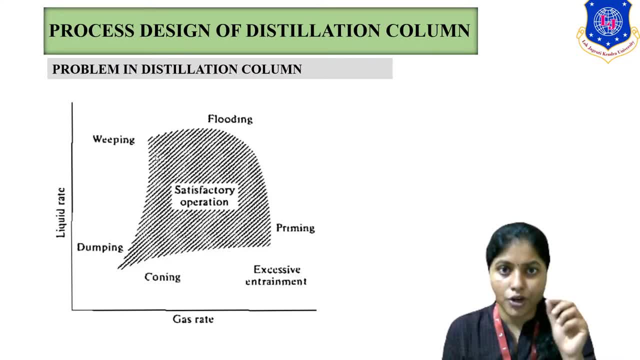 That is, that it will pour the liquid droplets outside the column And the last one is weeping. In the weeping, the condition should be lower vapor and high liquid flow rate. Here the mass transfer will not take place because of the high liquid flow rate and low 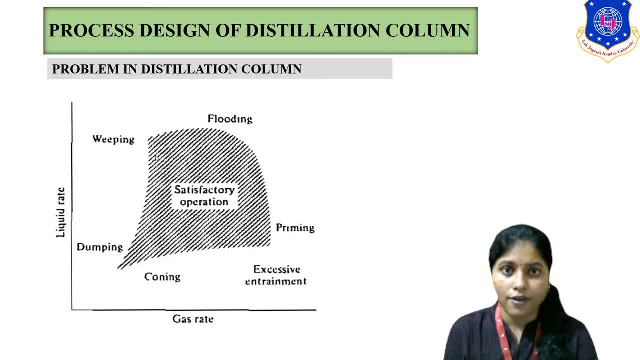 vapor, So it will pass from each sieves. So the gas flow rate is very less, While the liquid will pass from the each sieves. So the gas flow rate is very less, While the liquid will pass from the each sieves.